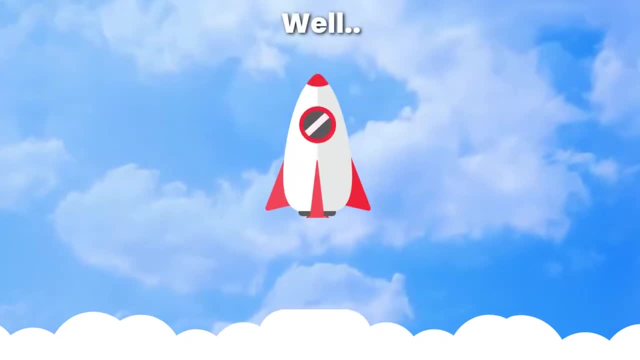 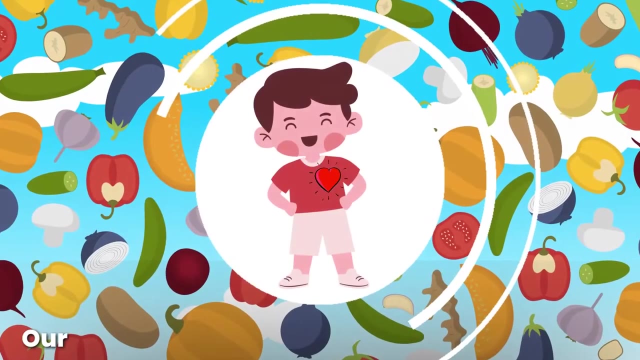 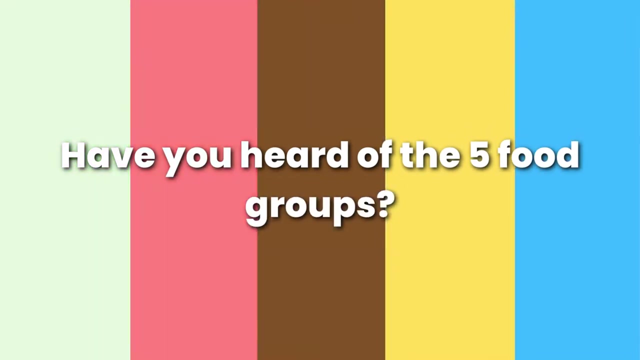 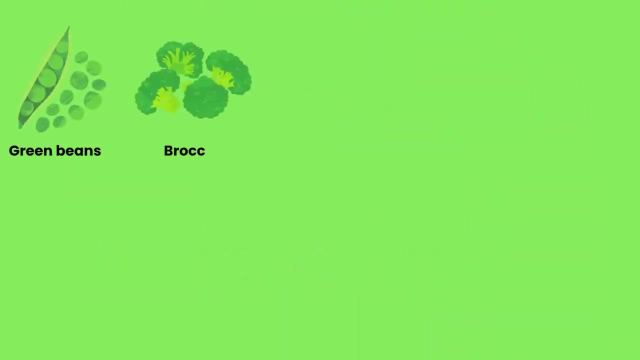 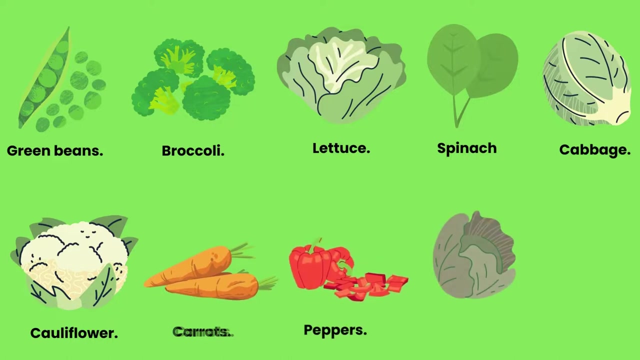 if you tried to launch a rocket without fuel, Well, it wouldn't get very far. Our body needs food, just like a rocket needs fuel. Have you heard of the five food groups? Let's start with vegetables: Green beans, broccoli, lettuce, spinach, cabbage, cauliflower, carrots, peppers, purple cabbage and asparagus. 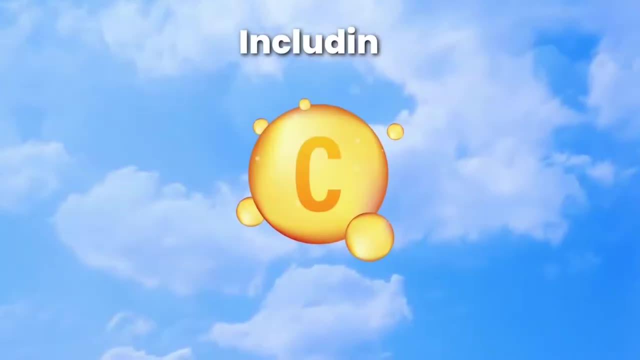 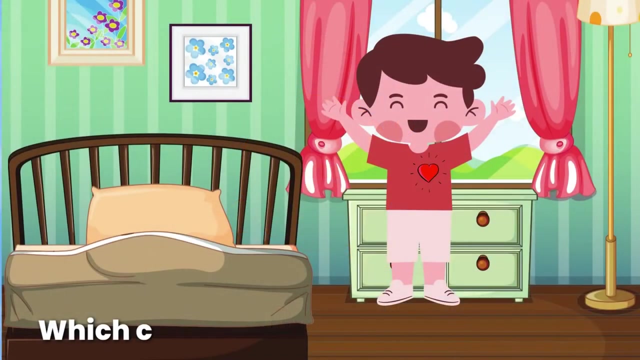 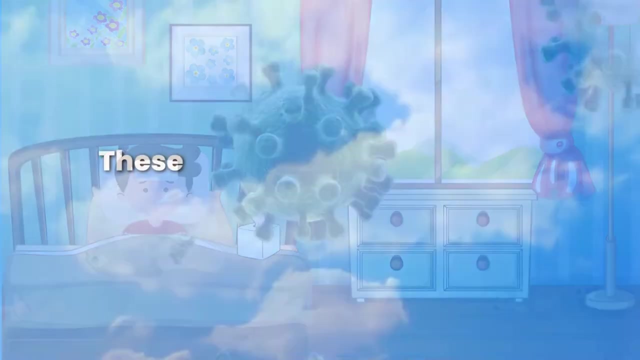 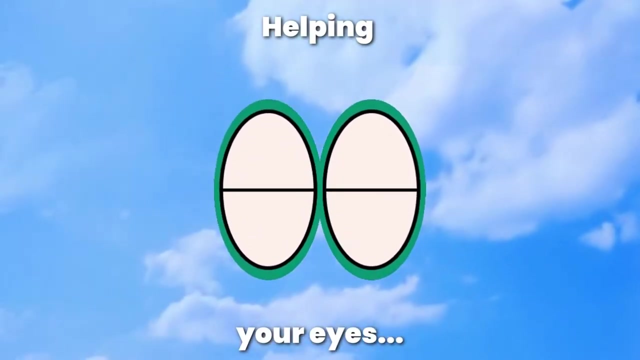 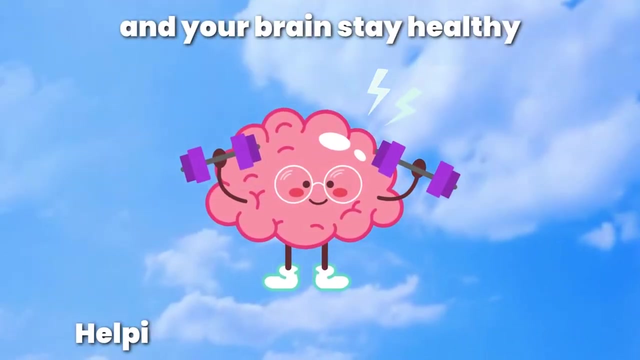 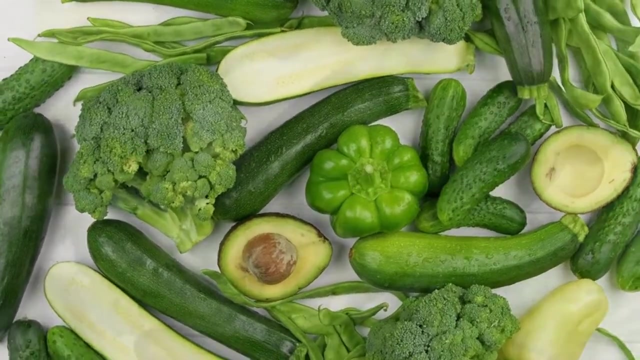 Vegetables contain lots of vitamins, including vitamin C and vitamin E, which can boost your immune system, keeping you from getting sick. these vitamins help your body in lots of ways, helping your eyes, skin and your brain staying healthy, helping you grow big and strong. the green and the vegetable, the better it is for you. fruits. 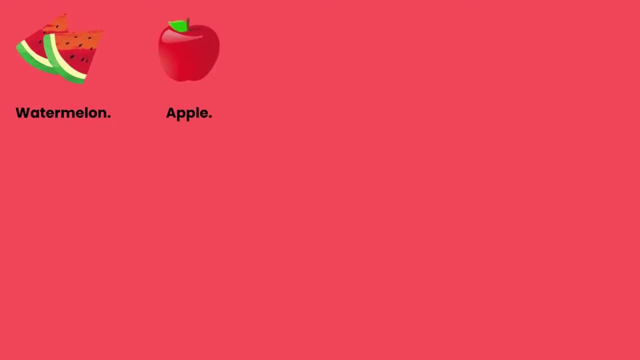 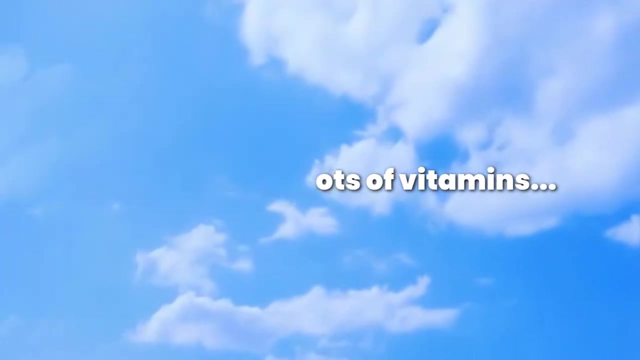 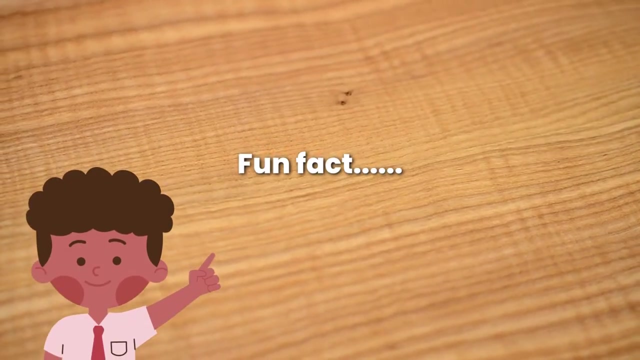 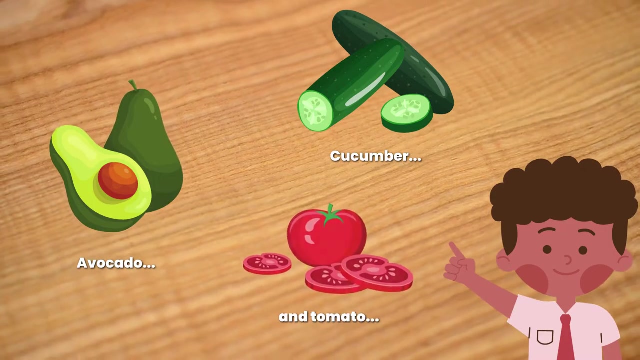 watermelon, apples, strawberries, oranges, peewee, raspberries, blueberries, pears and Fruits contain lots of vitamins, including vitamin C and vitamin K, Helping your bones, your teeth and your heart stay healthy and strong. Fun fact: Did you know that avocados, cucumbers and tomatoes are all actually fruits? 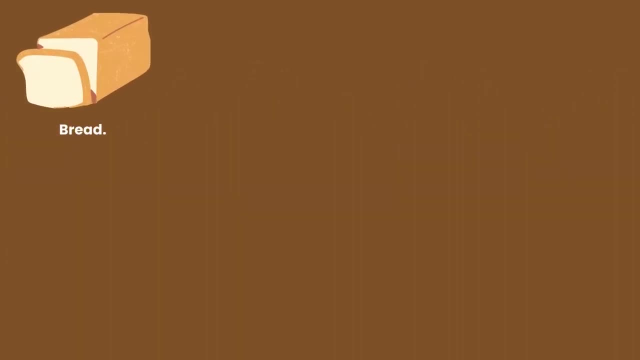 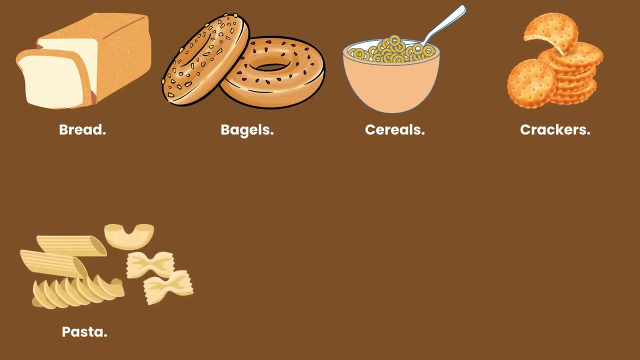 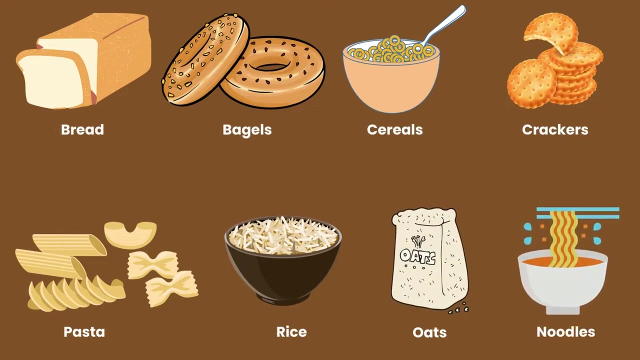 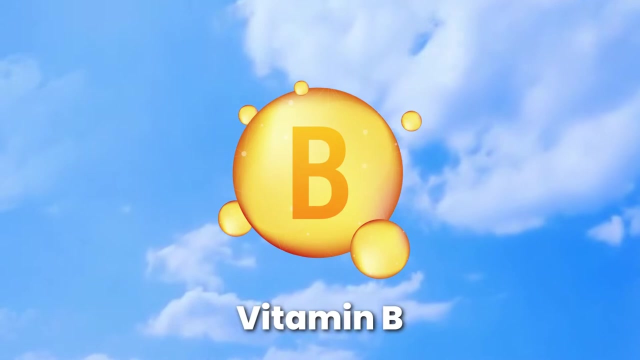 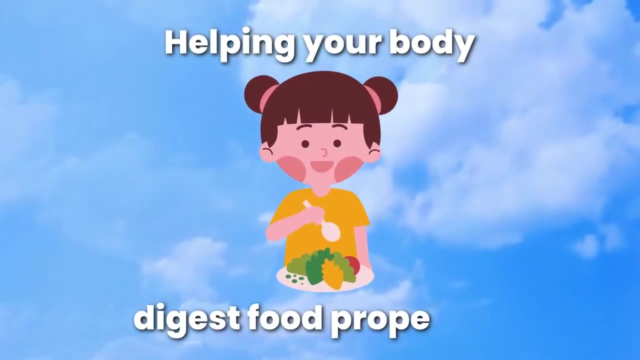 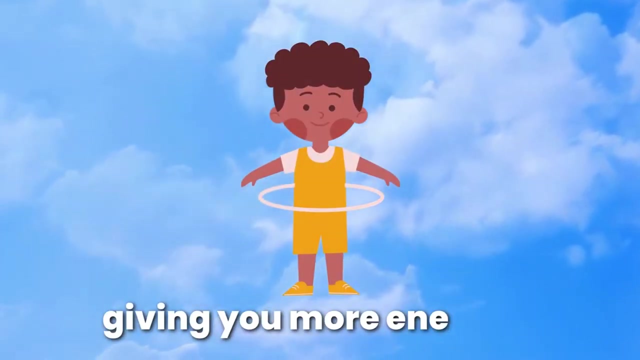 Grains, Bread, bagels, cereals, crackers, pasta, rice, oats and noodles. Grains contain vitamin K and vitamin B, carbohydrates and fibre, Helping your body digest food properly, boosting your mood, giving you more energy and keeping your heart healthy. 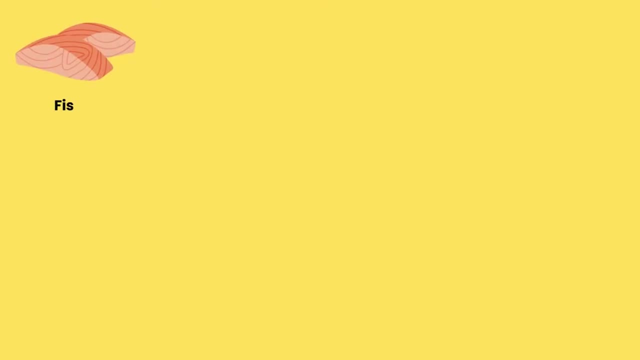 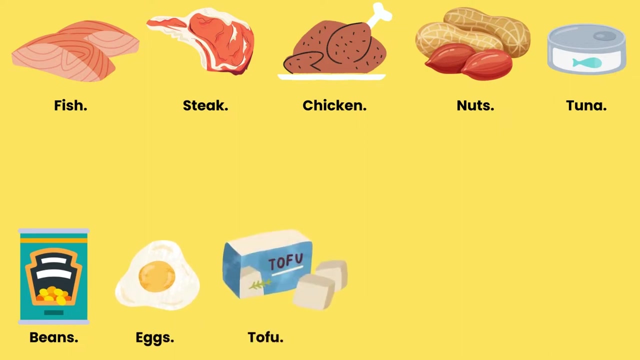 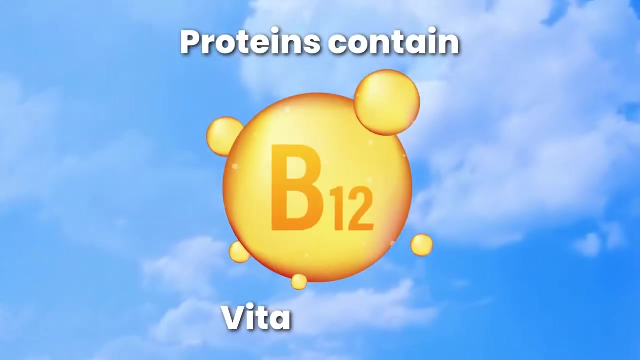 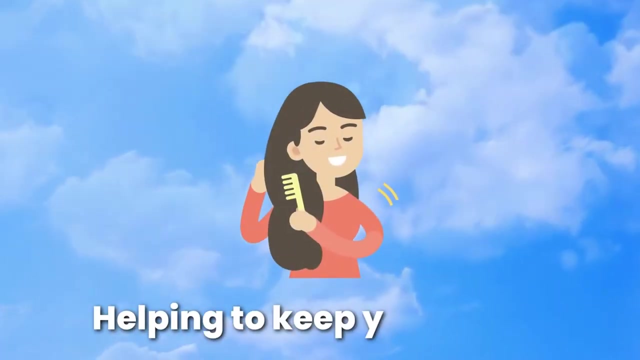 Protein: Fish, steak, chicken, nuts, tuna, beans, eggs, tofu, sausages and lentils. Proteins contain vitamin B12 and vitamin D, Helping you keep your hair, nails and muscles stay strong and healthy. Dairy: 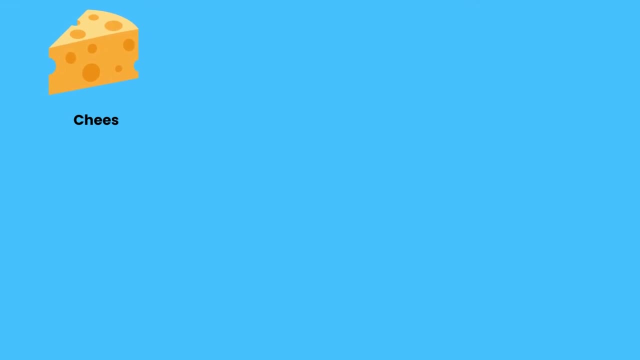 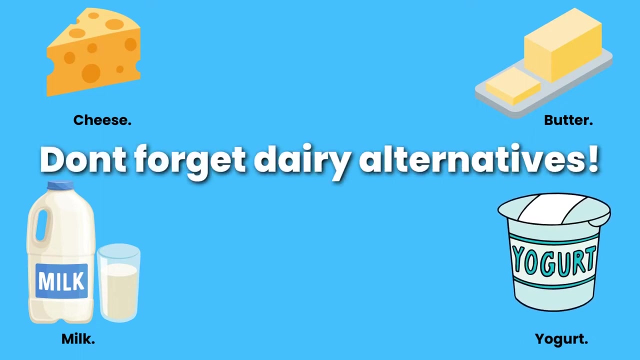 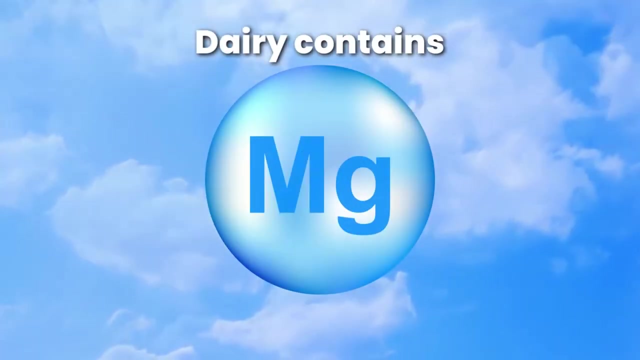 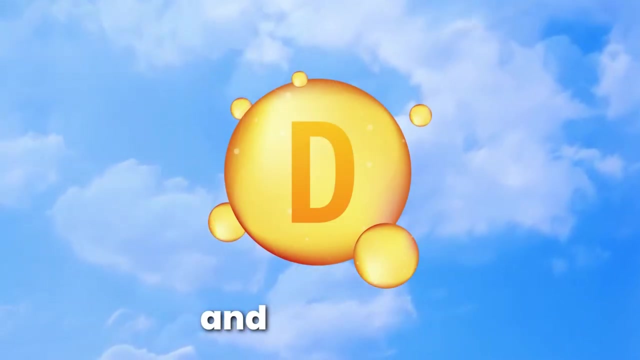 Cheese, butter, milk, yoghurt. Don't forget the dairy alternatives: Oat, milk, vegetable butter, dairy contains magnesium, calcium and vitamin D, Helping your bones grow strong, Helping you stay calm, Helping your teeth stay strong And even helping you sleep. 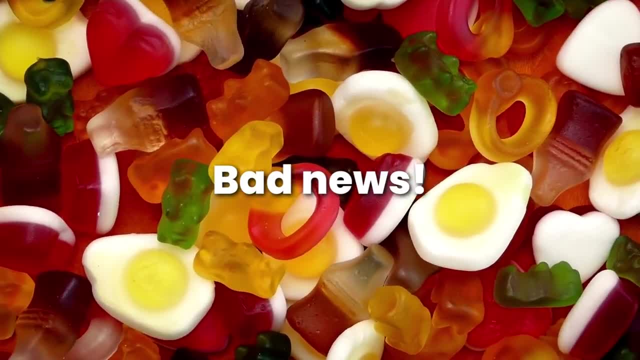 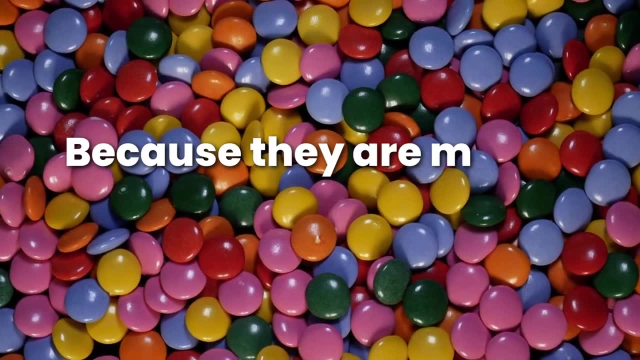 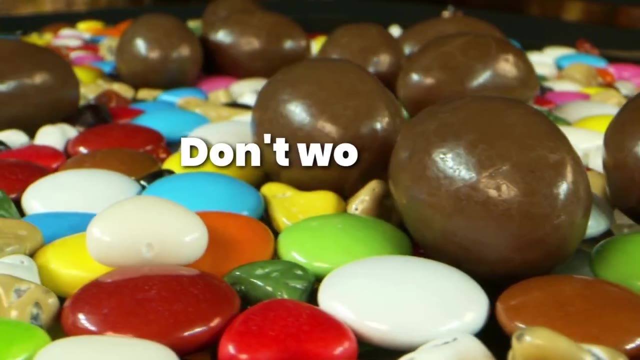 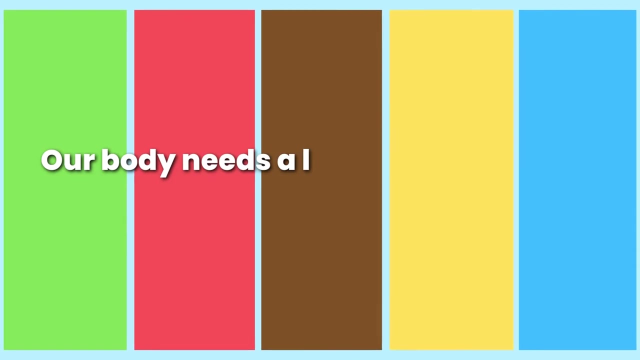 Uh oh, Bad news. Sweets don't fit into any food groups Because they are mostly made out of sugar And they don't really have what our body needs. Don't worry, You can still have them now and again. Our bodies need a little bit of each food group every day. 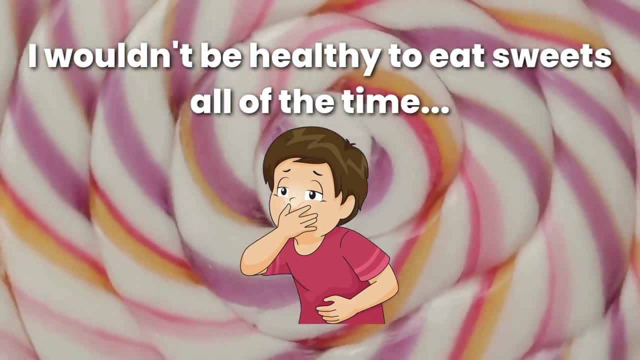 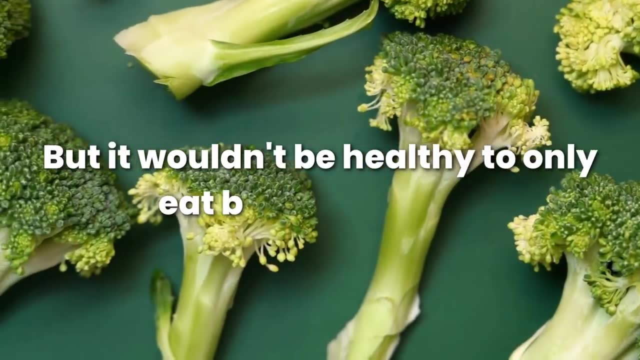 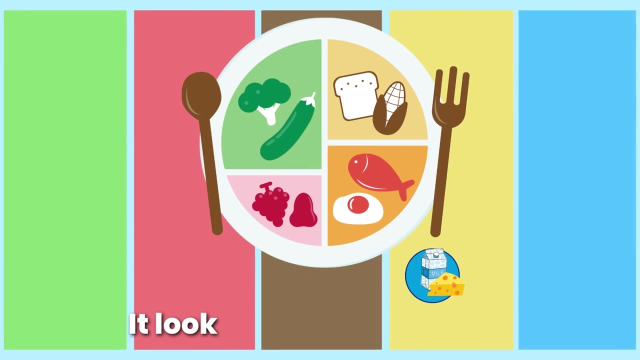 It wouldn't be healthy to eat sweets all of the time- That would make you sick. But it wouldn't be healthy to only eat broccoli either. It's all about balance. It looks a little bit like this: Can you remember the five food groups? 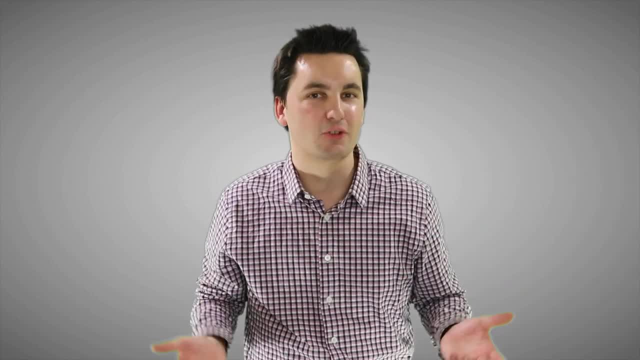 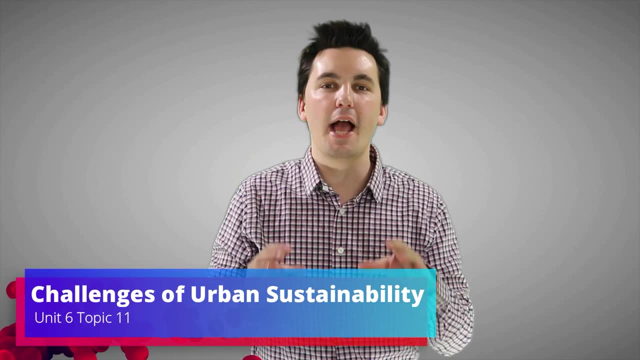 Hello there, geographers, and welcome back to another topic review video on the Mr Sin channel. Today we're going into the last topic review video for Unit 6.. We're going to be looking at Unit 6,. Topic 11, Challenges to Urban Sustainability. 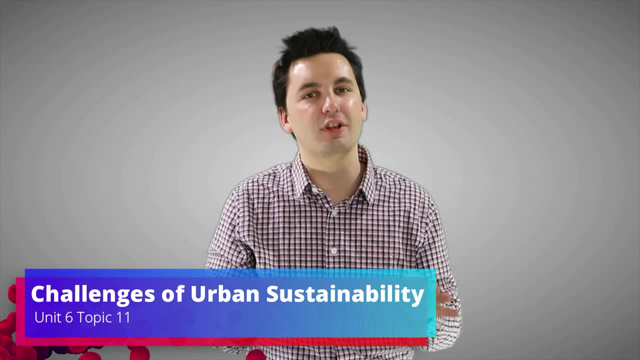 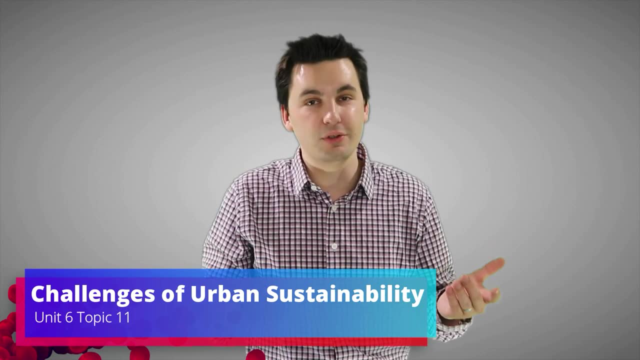 Now, while this video might be the last topic review video, it is not the last Unit 6 video. I also have a Unit 6 summary video that goes over all the major concepts in this unit, And not only does the video cover everything you need to know for your AP class, but also the national exam. 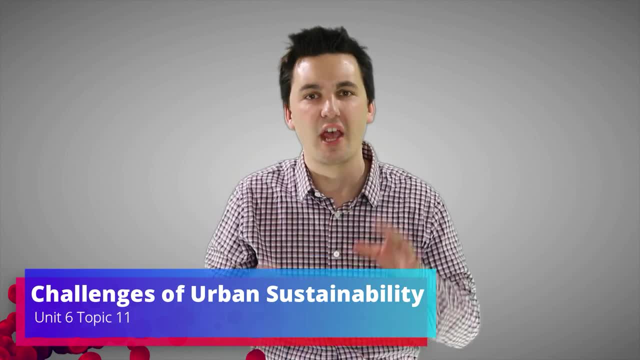 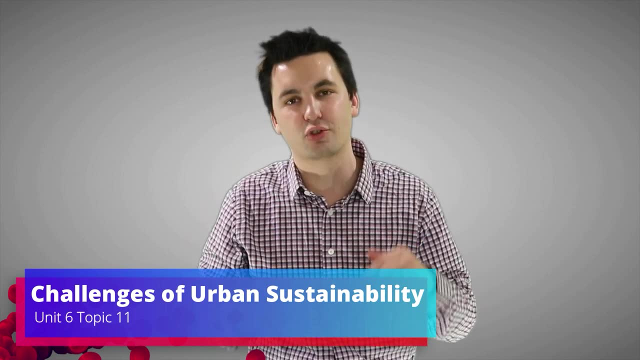 it also comes with study guides, answer keys, practice quizzes and much more, And it also covers all the other units in AP Human Geography. You can find a link to this awesome resource in the description of this video, But first let's go through this last topic review video, then go check out that resource. 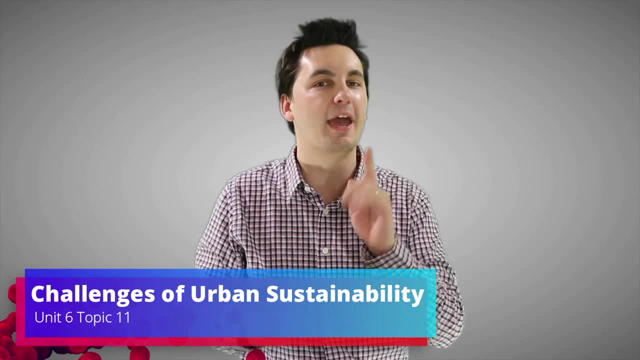 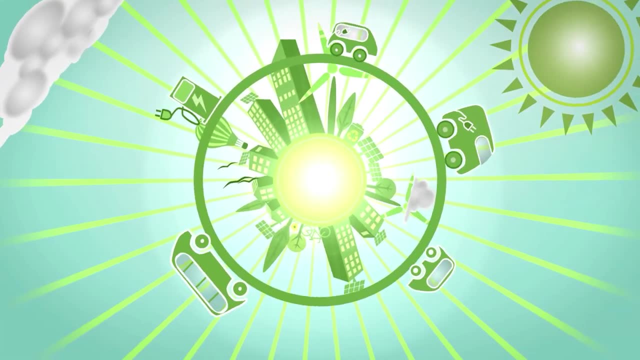 and then make sure to watch the unit summary video. That way, you don't miss out any information that you need to know for your class. So, like we've talked about on this channel before, sustainability is all about being able to use our resources. today, 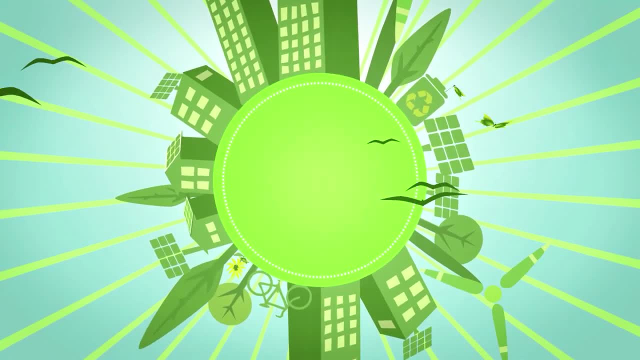 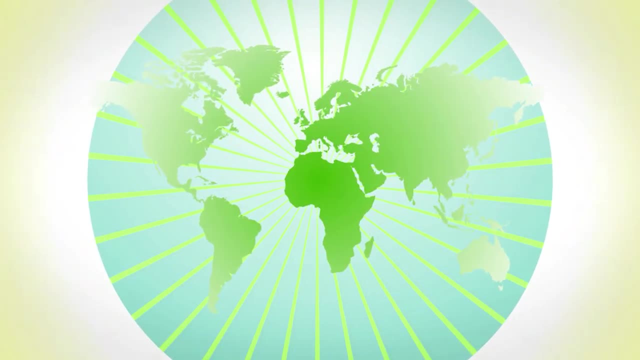 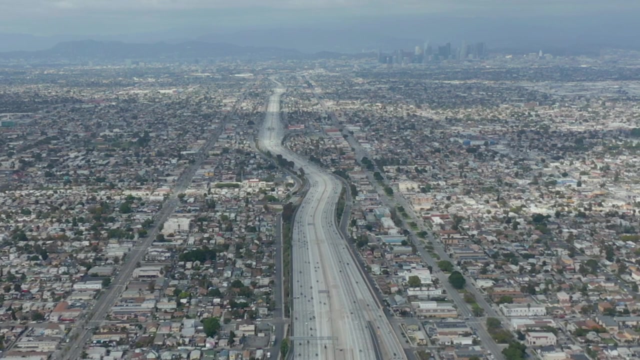 to satisfy our wants and needs While making sure that future generations can do the same. And when cities experience things like urban sprawl, they risk their long-term sustainability. Cities' landscapes start to destroy the natural resources they depend on. As cities continue to grow and expand outwards, they may experience more costs, more services. 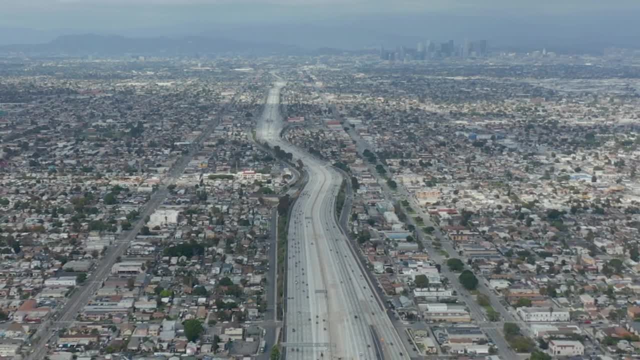 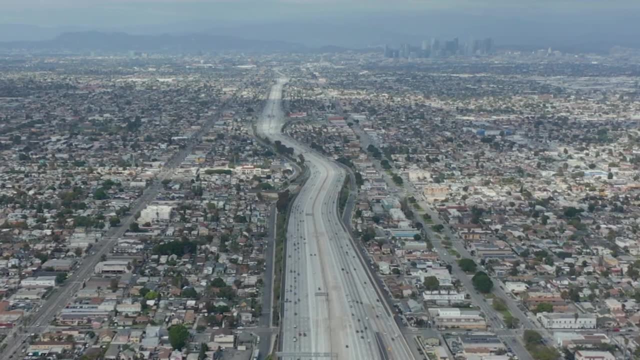 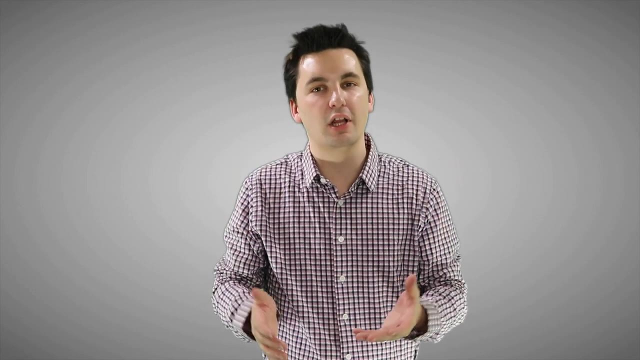 that will be needed to cover the growing city, Which will increase taxes, reduce the amount of affordable housing and cause stress, reducing the standard of living For people in the city. We could also see health concerns arise in densely populated areas As cities continue to grow and expand if they don't utilize urban planning correctly. and create a sustainable city, we might start to see the population grow at a faster rate than the infrastructure can keep up. This could reduce the amount of education, healthcare facilities. It also could reduce the amount of clean water, sewers or even electricity to the residents.